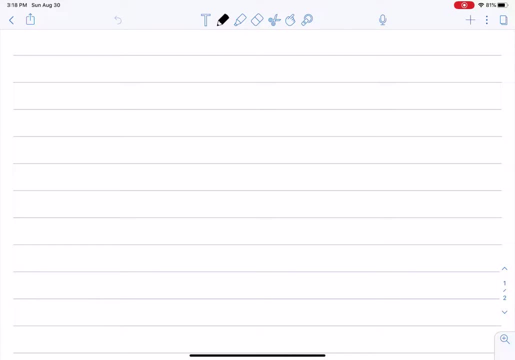 I will now talk about one way of representing this data structure that captures disjoint sets. And the first representation is a simple representation using linked lists. So linked list representation of disjoint sets. Let's talk about one set in the set of disjoint sets. So imagine that we are talking about set SI that has A, B, C, D in it. The way we are going. 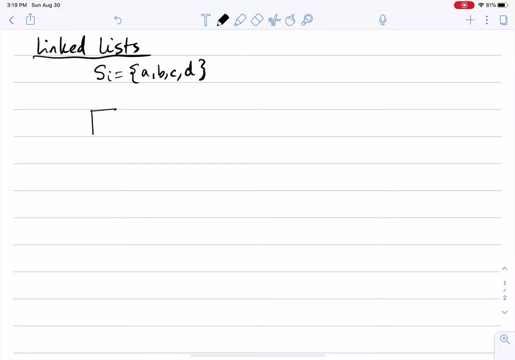 to represent. this is a linked list. The linked list is going to have the main object here and the main object will point to head and to the tail of the list itself. So now, since the set has four elements, we are going to have four additional objects in the list. 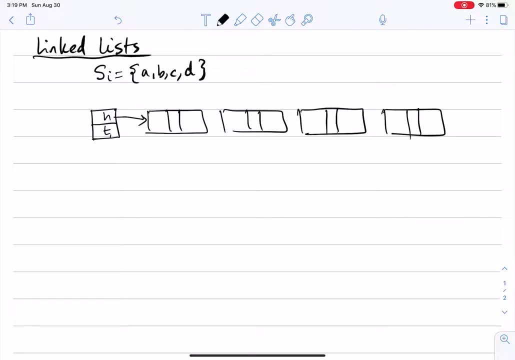 The head is going to point to the first element. The tail is going to point to the last element here. Okay, so the first element is A, Then B, then C, then D. The first one in the list is always the representative of the set. So if this: 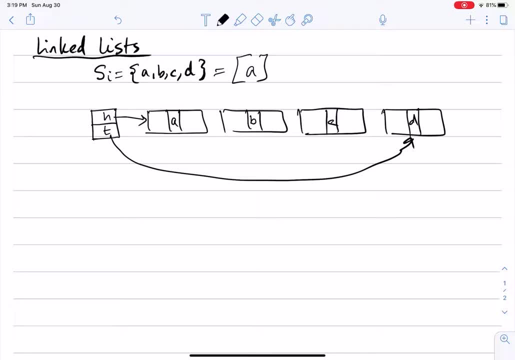 set is represented by A, then that's the element there. The last element in each object is going to be to the next element here. So the next of A is the object that has B, Next of B is the object that has C. Next of C is the object that has D. Next of D is nil nothing. The first element here. 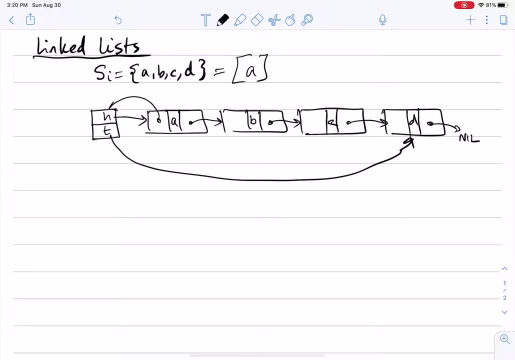 is going to point back to the main object of the list. Okay, so this is the main object of the list. This is it's going to point to the first one here. Okay, and so this is really a linked list representation of a set. Now imagine that. 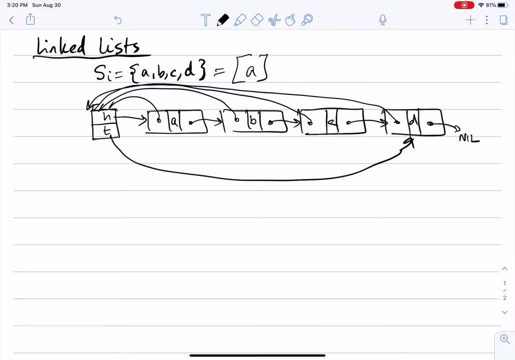 I want to create a list, a new list with one element, So the operation make set. If you think about the operation make set with element X, all we are going to do is create that object for the list with the head and tail. 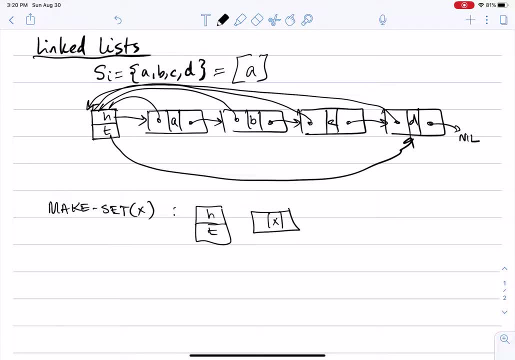 So we are going to create an element for X itself. The head is going to point here, the tail is going to point here: the same element, because the list has one element in it. Then this pointer here of X will point to the main element or main object of the list And the next is nil. So it's really 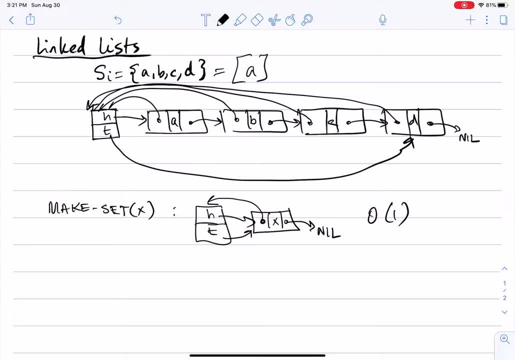 just all of one operations to make a set. Okay, what about find set? If we want to find set, and it's very easy to do, we're going to do it with a set. So if we want to find set, and it's very 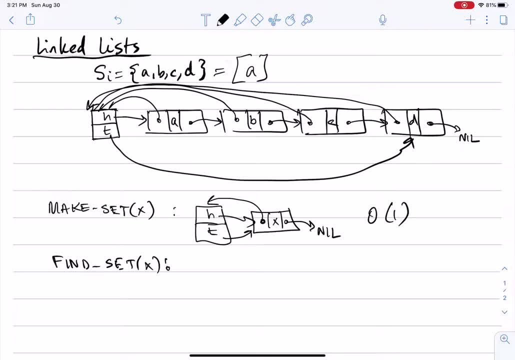 important here to to pay attention to what i'm going to say here. mix: find set x. i am giving you information, i'm giving you a pointer to that element x in the set. all i'm asking you is to find me the representative of the set to which x belongs. so i'm not asking you to go find x in the 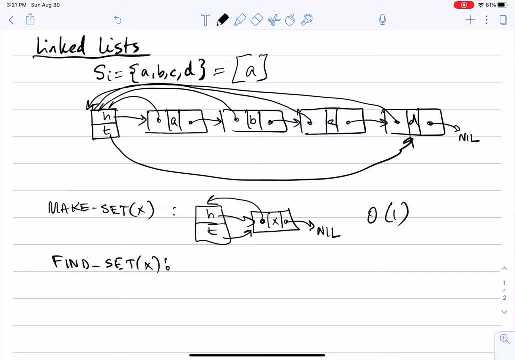 list and then find the representative. i am giving you the element x, i'm giving you a pointer to that element x and i'm saying: find the representative. so imagine that this x i want to do. find, for example, the element c, and so i gave you a pointer to c here. i said this is the element. 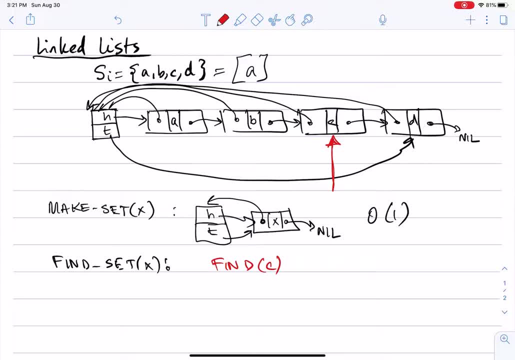 that i'm giving you. can you tell me what is the representative of the set to which c belongs? well, it's very simple, because now you can just follow this, this pointer from c you can point, you can follow it to the main object of the list and from the main object you follow the head. 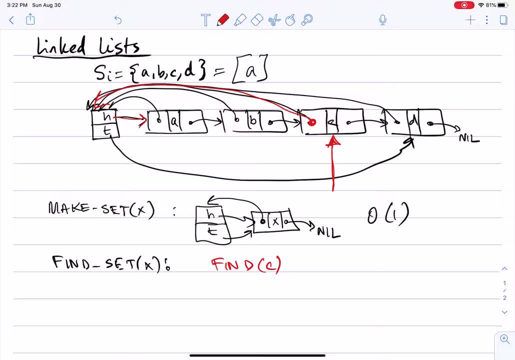 point lines. it's gonna take us to the first object. I look there, I find it's a, so I will say it is a. okay, so the representative of the set to which C belongs is a. if you think about this, it's also of one operations, because we need to follow two. 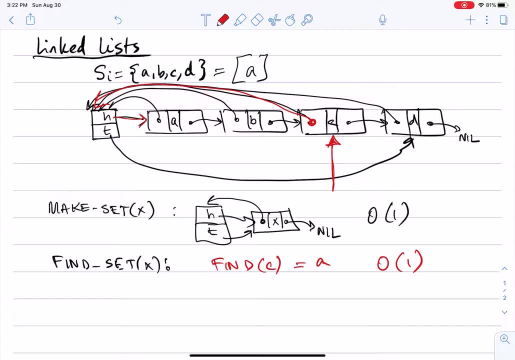 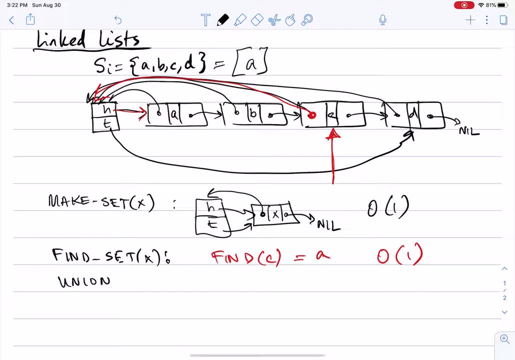 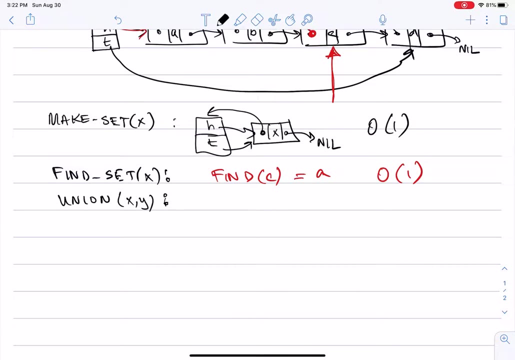 pointers. for any element you need to follow two pointers, really, okay. now, as you can imagine, the union will be the more costly one. so here I want to do union of two sets and let's think about how union would work. so imagine that we have, we have these two sets here and I'm not. now I will basically draw them like: 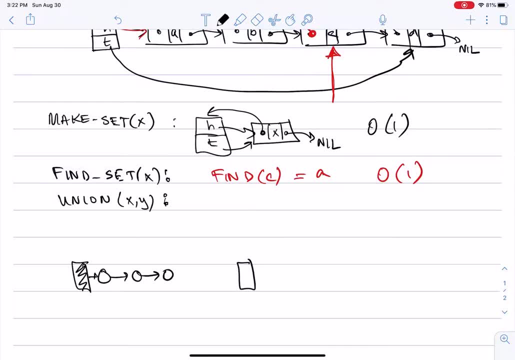 this, and so the first one corresponds to three elements and the second one here has as a set that corresponds to five elements, let's say okay. so of course we have these pointers, but I don't need to draw them in every case. okay, so suppose I want to take the union of these two sets here, or the unit I want to. 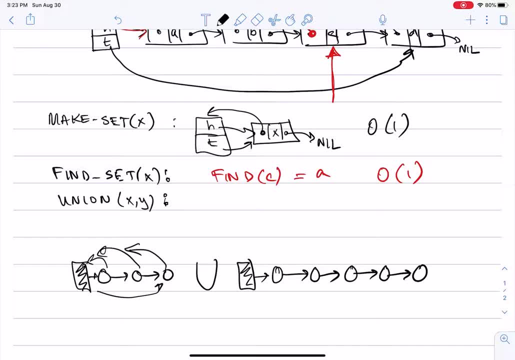 take the union of the two sets and the result should be a linked list that corresponds to the, to the union of these two sets. so, if you think about it, the main, or the main, operations I need to do are the following: well, since I will take the union, we will create one list, so we don't need these two objects for the the. 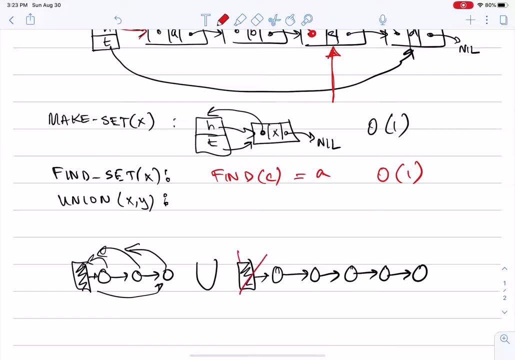 main, the, the two main objects for the list. so I need to get rid of this one. okay, so we need to get rid of this one. this is one operation here. second thing I need to do is that the next of the last one from the first list is now the. 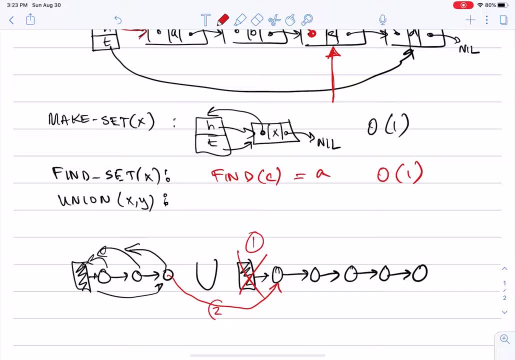 first element in the second list. this is another another operation here. the tail of the first list is no longer the tail that that originally was there. no, now the tail is the tail of the second list. okay, so this is a third operation here that we need to do, and it's very easy to. 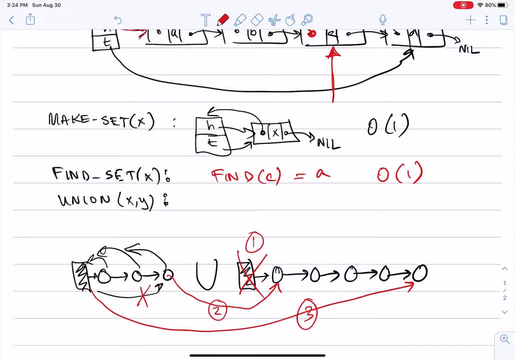 find it, because the tail would actually go to the tail of the main object of the second list. so third operation. so these are the, the easy ones, or the, the operations that are not time consuming. but what is time consuming is that we have these back pointers from every element in the list that need to point. 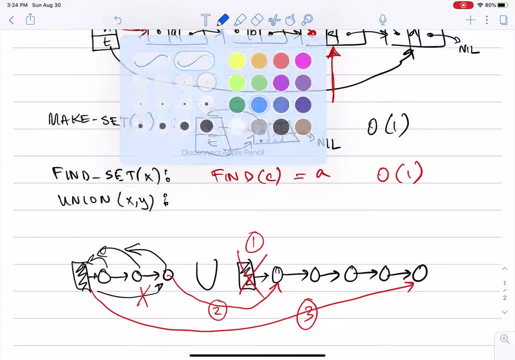 back to the main object. so now I need to update this back pointer to go all the way to this object here, okay, and we need to update this, i need to update this, we need to update this. we need to update this here, okay. so, if you think, 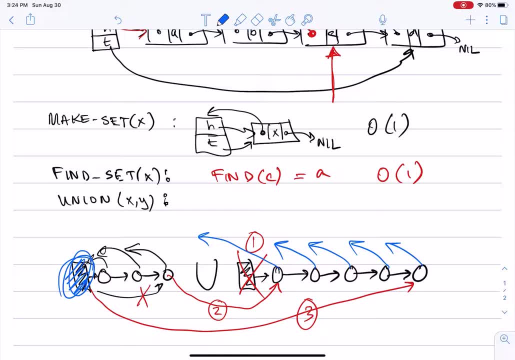 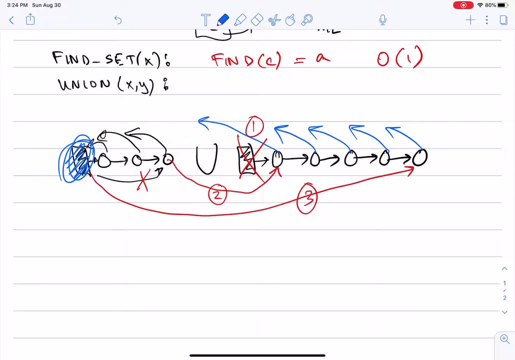 about it now, we need to do five operations to update all these ones. now, if we think about it, if you think about the three applications i illustrated, which is the equivalence classes, the connected components and and the minimum spanning tree, if you think about it, the way the algorithm worked is: first we started, started individual sets, each of which has one element in. 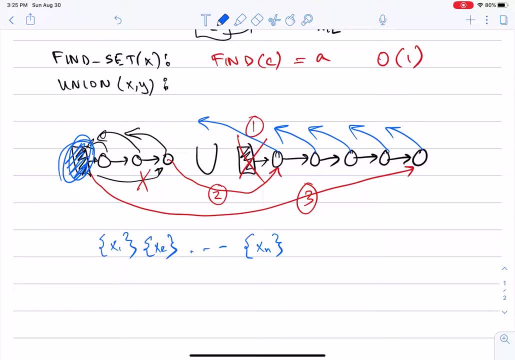 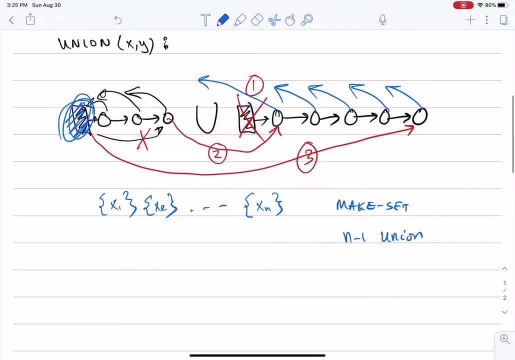 it okay. so we started n sets. this is where we called make set. okay, and there are in n sets there, each of which has one element, and then after that we, in the worst case, we could call n minus one union operations. okay, now the n minus one union operation combined. how long do they take combined? how long do they? 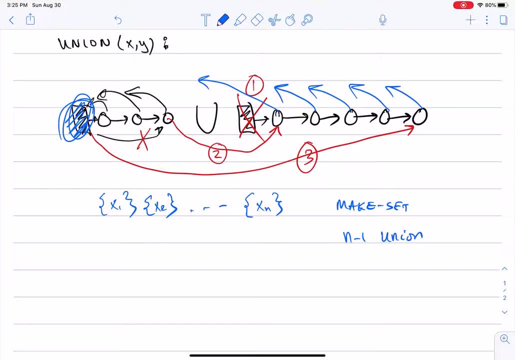 take. well, imagine that first i have, i have a list with one element. i want to do a union with a list of another, another list with one element. so if i want to do this, it's okay, i need to update this element here, but the result is now a list with two elements, right? so this is the union. 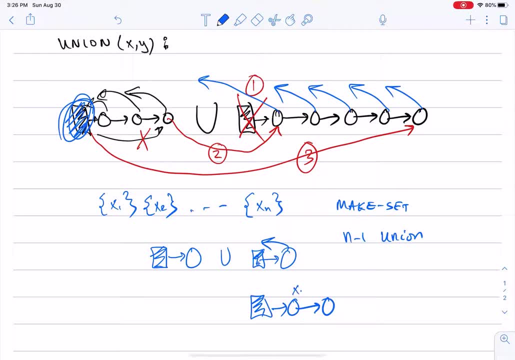 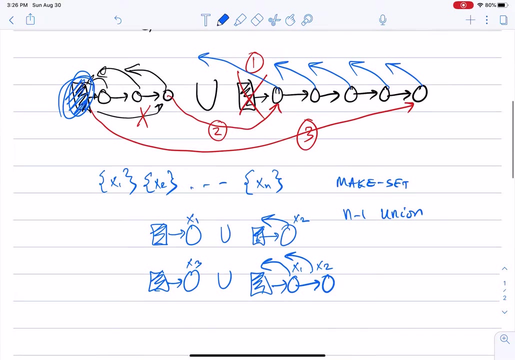 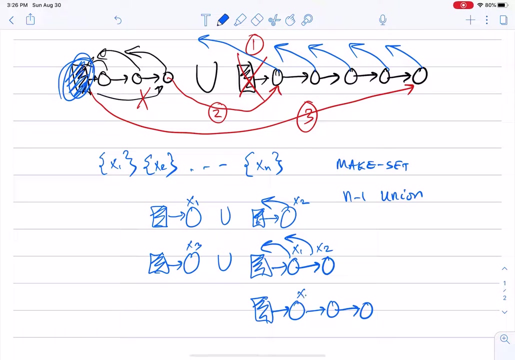 suppose now. so suppose this: this now correspond to x1 and x2. this was x1 here and x2, and suppose now i want to take the union with a list that corresponds to x3. okay, so now i need to update this one and this two here and the result now will be x1, x2, x3, and suppose i want to do the union with. 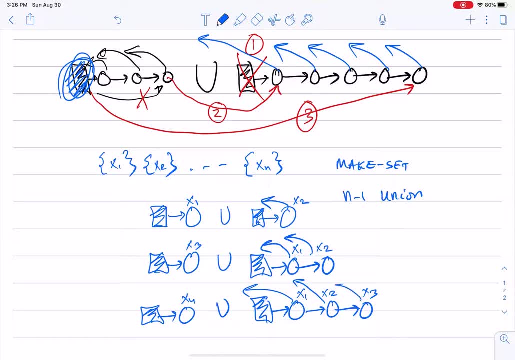 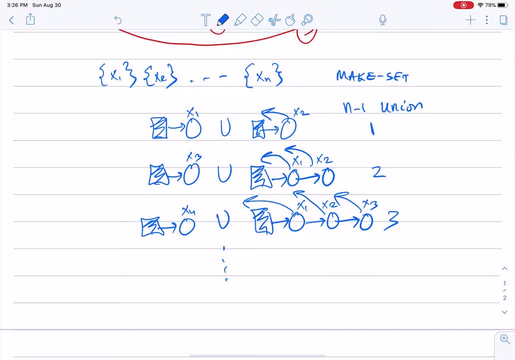 xn. now i need to update three of them here right. so now we need to do one. one update here, two updates here, three updates here after some point again, in the worst case- i'm drawing a worst case scenario here- we might have this situation where we have x1, x2 all the way to xn minus one, and here 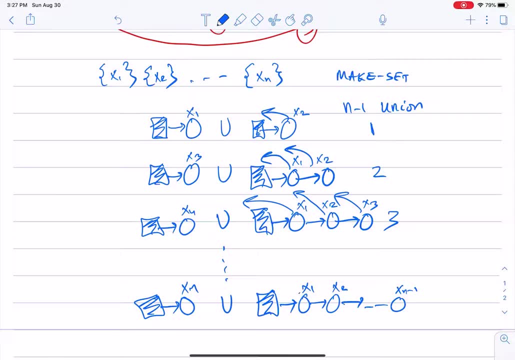 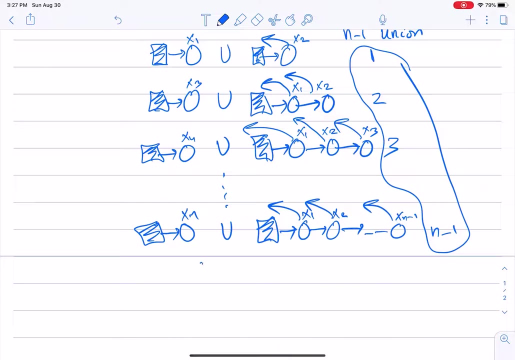 we have this list with one element, xn. we need to update one, two, all the way to n minus one. so this is n minus one updates here. so the total number of updates we need to make is this: the sum of these numbers: one plus two plus three plus all the way to n minus one. and this shows us that 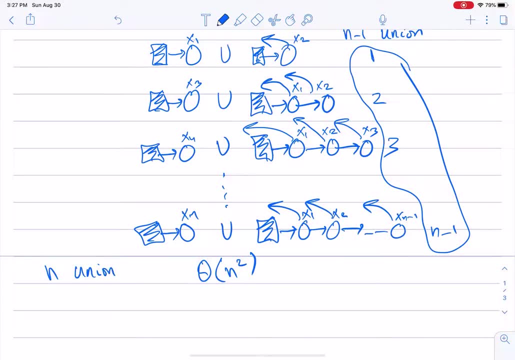 n union operations, or in this case it's n minus one. really, it's n minus one union operations. takes theta of n squared. now notice how i'm analyzing the running time here. i'm not focusing on one union operation because the algorithms that are working on these disjoint sets are always doing a sequence of. 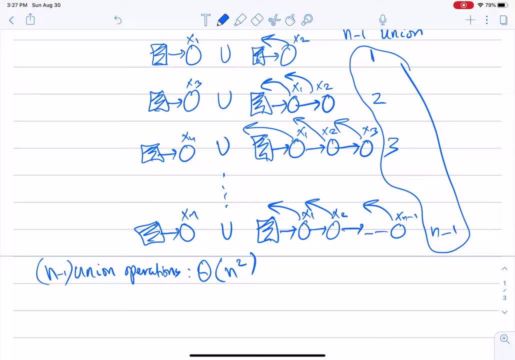 these operations of creating in the, you know, singleton sets with one element and then a sequence of union on them, and so on. so i am analyzing the total running time that n operations in this case, or n minus one operations would take. this is what we usually talk about, what we refer. 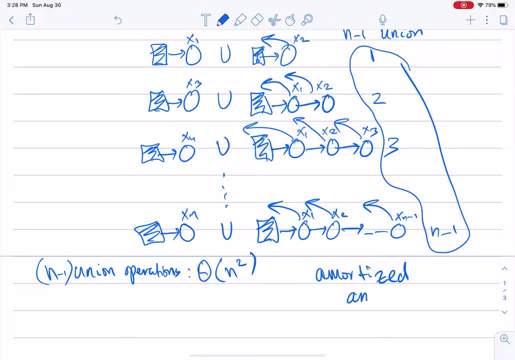 to as amortized analysis. okay, amortized analysis because now i can take that theta of n squared. i said: on average, how much does every operation take? i said, okay, if n of them is taken n squared, then each of them, on average, is taking n time. okay. 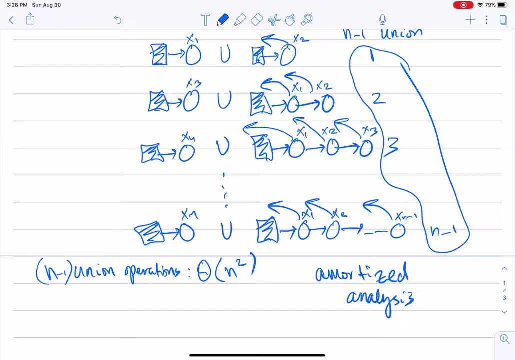 and this is the type of analysis we do when we work with this type of data structures, where we are talking about these disjoint sets, and almost all algorithms that are making use of them always consist of a sequence of such operations. we want to know, on average, or the total running time of 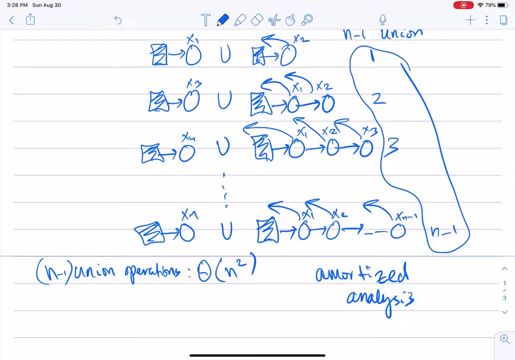 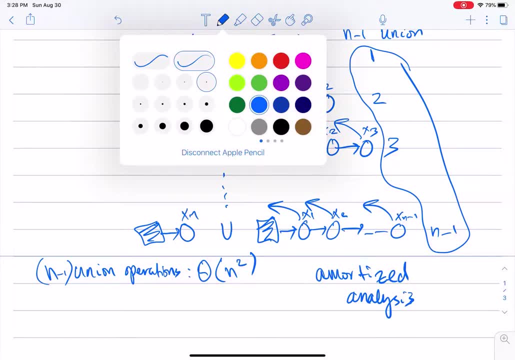 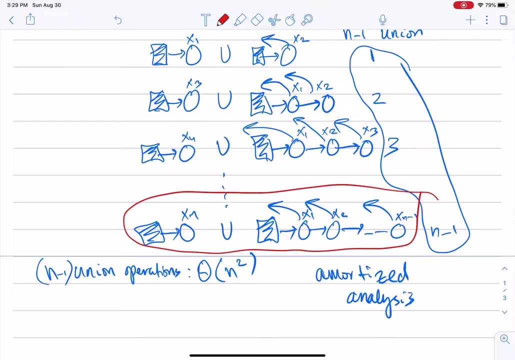 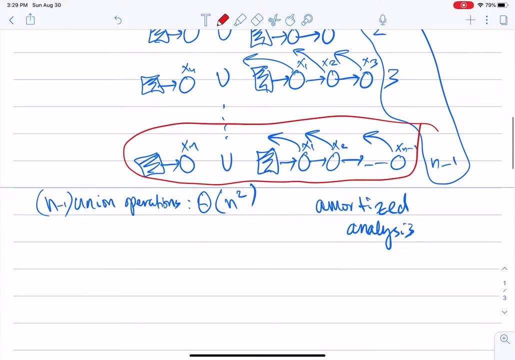 look at this. if you pay attention to what i just drew here, let's look at this, the last one, for example. so i chose to do the union of the list on the left has one element. the list on the right has one element. the list on the right has one element. the list on the left has one element. the list on the right has one element. 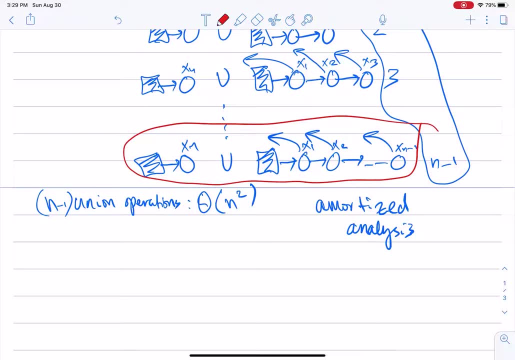 but the union is of course commutative. i could have done this. so this is x1 to xn minus one. i could do the union such that the shorter of the two lists is on the right. if i do this, the only the only update i need is just one, only one operation here, right. 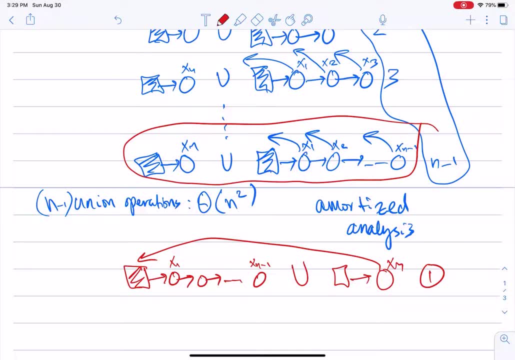 so this simple modification is basically the only thing i need to do is to update the list, basically saying, when you are doing the union and you are have the list, that correspond to two sets, and imagine that we are always updating the pointers for the list on the right when you 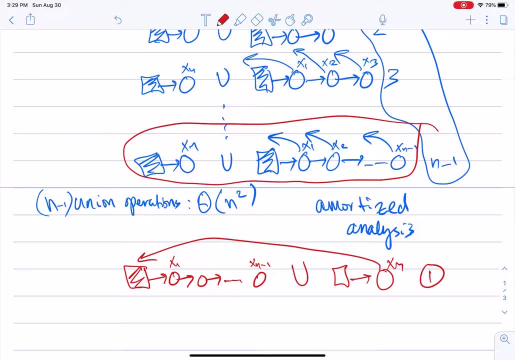 are doing the union, always update the pointers to the shorter of, always update the pointers of the elements in the shorter of the two lists. so if you are taking the union of two lists- one has 100 elements, one has 50- you update the pointers on the list. 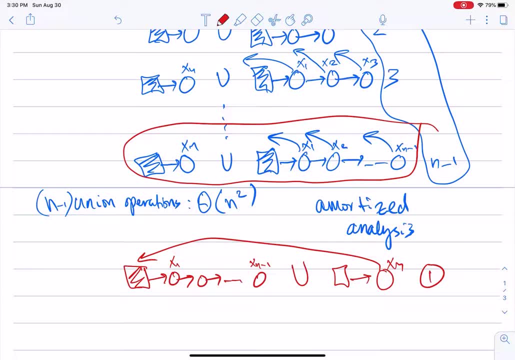 that has 50 elements. how do we know that? we can add very simple modification. we can add just one number to the main object of the list that says how many elements are in that list. so when you ask me to do union of two lists, i look at how many numbers are in, how many elements are in them, and i always 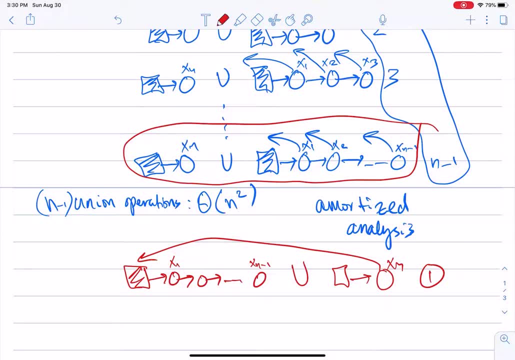 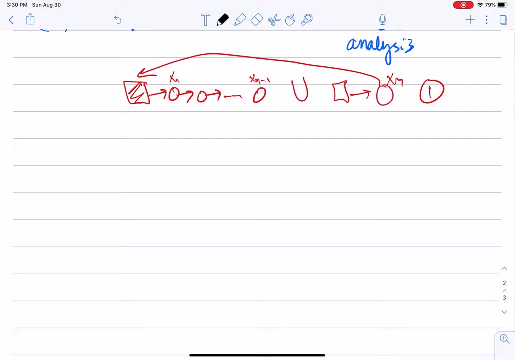 update the the pointers of the shorter of the two lists. now, does this trick really result in shorter amount of time? and even asymptotically? the answer is yes. so if we think about it asymptotically, let's actually look again at n minus one, n minus one union. 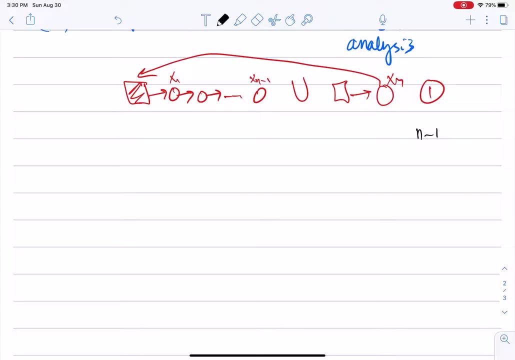 operations where we started with these in singletons, sets of individual, of single items in them, and i want to do the union okay. so if i want to do the union, the first thing i would do- and i will always draw the the longer of the two lists on the left and the shorter on the right. so first, 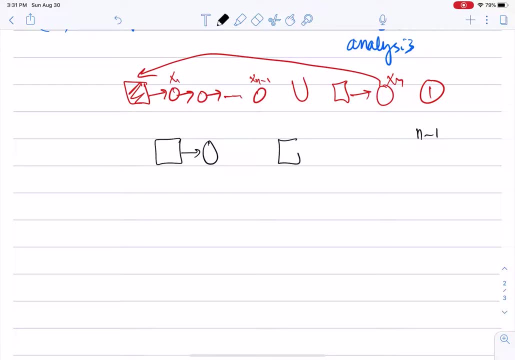 thing. imagine that i have two lists that i want to take the union. okay, and let's focus on one element, x- here. if i want to take the union here, i need to update x. so this will be the point of: x is going to be updated. this is one operation. now i created a list that has two elements in it. 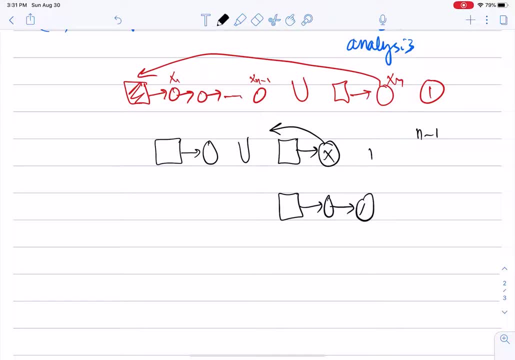 the list has two elements in it and x is one of them, and i'm doing union here with some other list and i, 과А Iranian, will say that the pointer to x is going to be is going to be updated. if the pointer from x is updated, then the length of the list on the left must be at least as long as the one on the right. 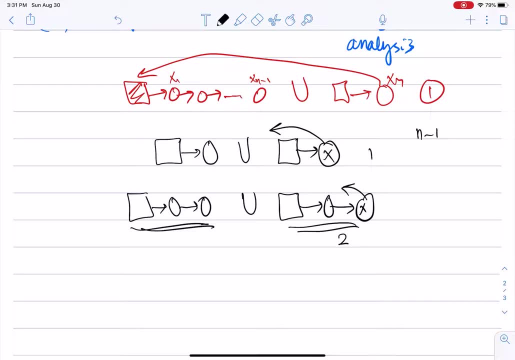 right. so if the one on the right has two elements- and again i'm focusing on the circles here- the one on the list has to have at least two elements, because if it had fewer than two elements, then i will not be doing the union like this. i will be do. i will be swapping the order of 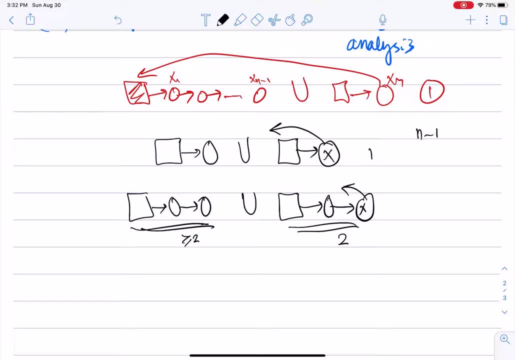 of these two sets. so this now x. i will update the the pointer to x to the left. but what would happen once i take the union of these two? the one on the right has two elements, the one on the left has at least two elements. so now i created a list with at least four elements in it that has x here. 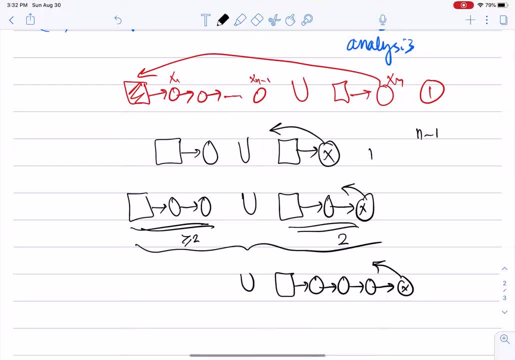 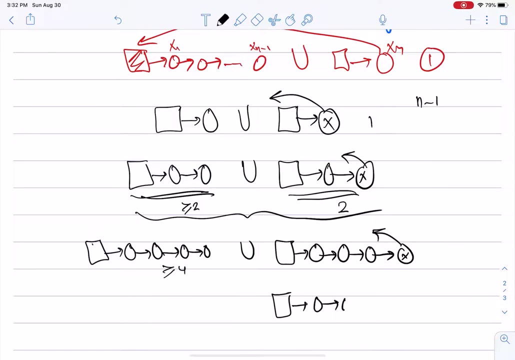 and if i want to do a union- and the pointer from x will be updated- then the list on the left has to have at least four elements in it. you well, at least four. it could be more okay. now, once i'm done with this, i will create a list that has. 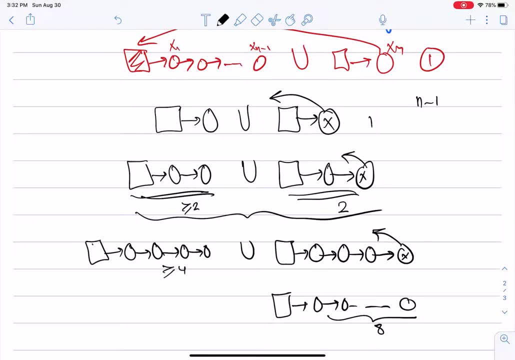 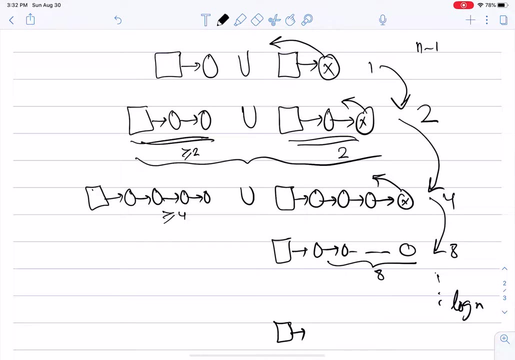 eight elements in it. so look what happened here. the result from here was a set that has two elements. the result from this was a set that has four elements. from here it's eight and if you think about it, after log n operations you are going to get to a and at most after log in. 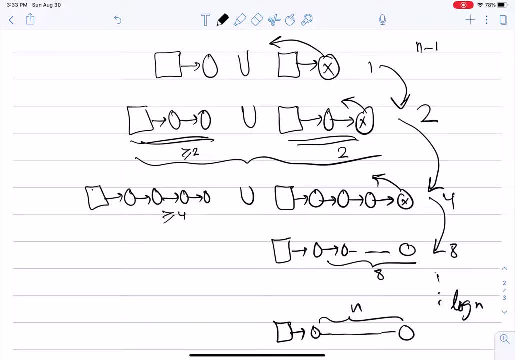 operations, you are going to get to a list that corresponds to n to n uh elements in the set. okay, so what this analysis is telling me that the pointer this, the back pointer from x to the main element or main object of the list, will be updated at most, at most log n times. 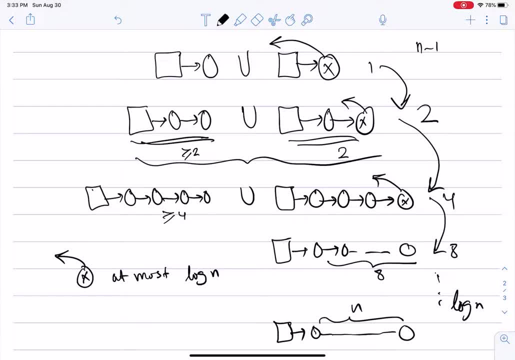 okay, so a back pointer. under this simple modification to the algorithm, where we always update the pointers in the shorter of the two last, the back pointer of an of an individual element in a list will be updated at most log n. in the worst case we need to update the the. 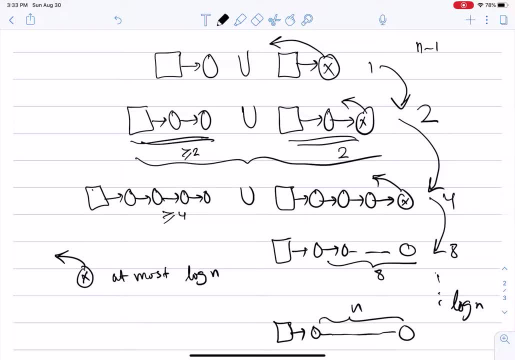 back pointers for, in the worst case, to something on the order of n elements. right? so if i'm, if i'm taking the union of two of two lists, for example, one is n over two elements, one n over two- i need to be doing the update for n over two elements. so if, for every element we do at most, 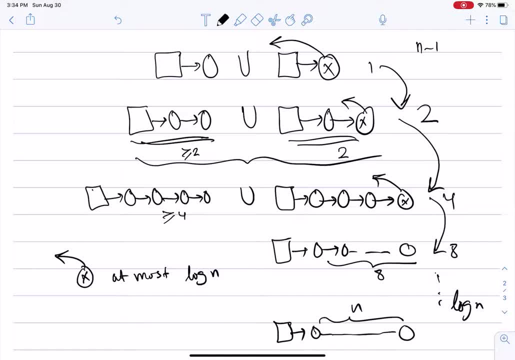 log n updates, and there is, there are, in the worst case in elements whose back pointer i need to update. then in union operations, in union operations will at most do n log n back pointer updates. okay, so this implementation is ordered by the specific intent of the student from the